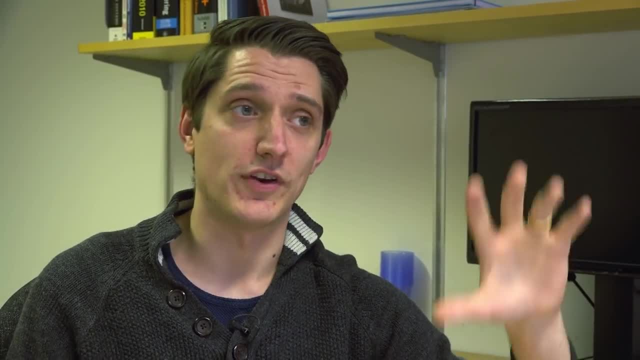 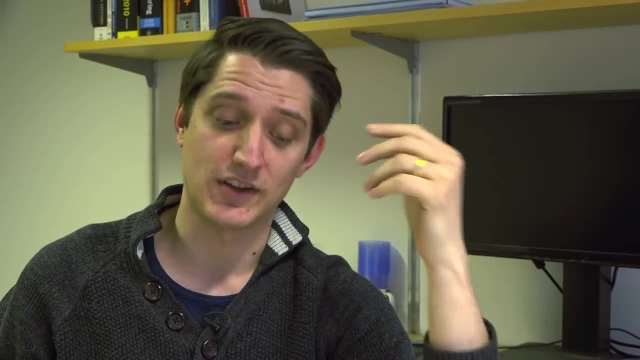 Route planning also comes in on things like routing. so if you've got a network and lots of routers, what's the best way to route those packets through which ports to get to your destination the quickest? So things like this. Now, Dijkstra's shortest path sees a lot of use in all of this. 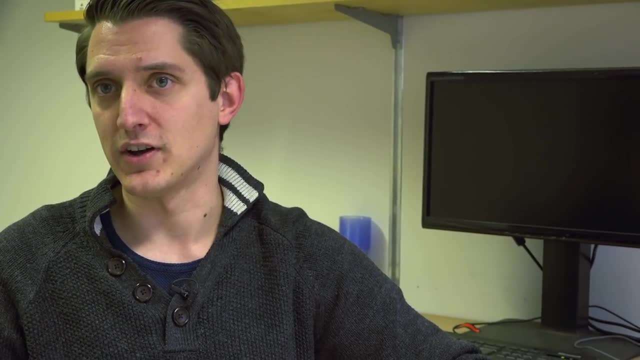 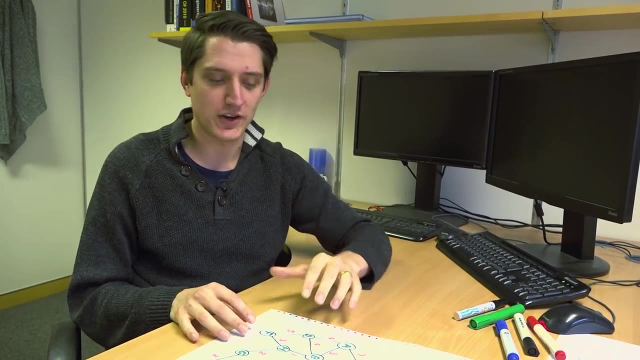 And extensions of it, so, for example, A-star search. So I've drawn out an approximation of a road system on this piece of paper. So we're going to use the analogy of roads for this one, because I think it's a good example of Dijkstra's shortest path. 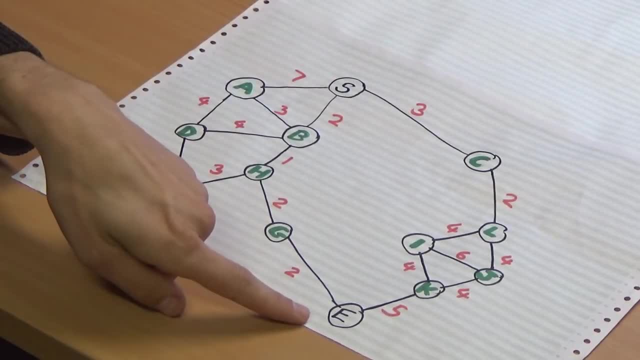 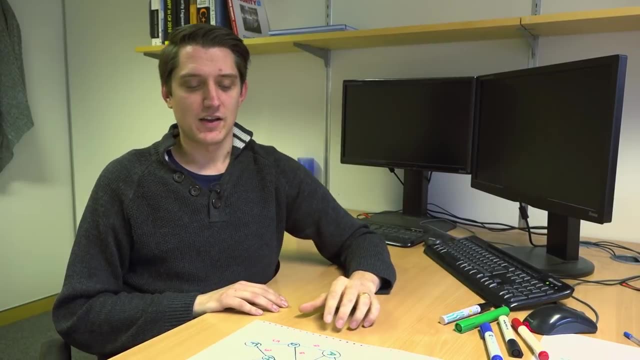 And we're trying to start here at S and get down to E. This is, broadly speaking, a small version of what a sat-nav does. when you say: how do I get there? Now, each of these nodes represents a different route. 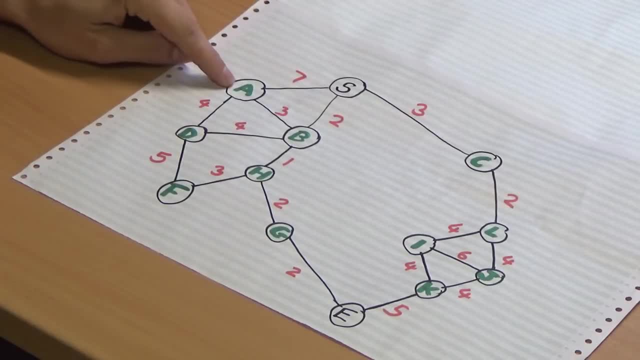 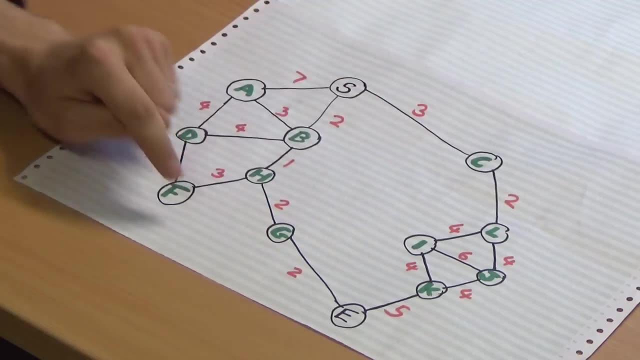 It represents a junction, So the vertices on the graph. so A could be a roundabout, B is a T-junction, doesn't really matter. Actually, B is more of a roundabout because it has four outputs. Anyway, each of these numbers represents how hard it is to get along that road. 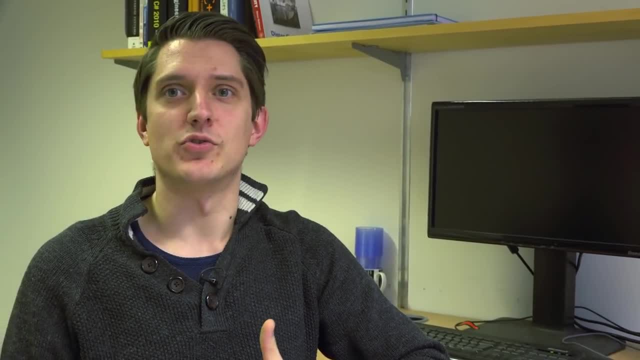 So that in real life would be, whether it was a motorway or a highway, whether it was a country road with a load of potholes, maybe there's a tree down it, and so you can't get through that road. 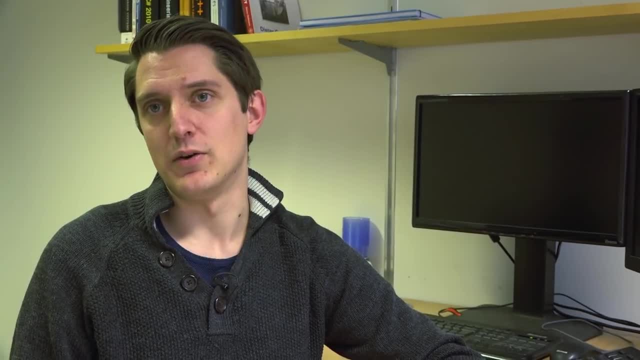 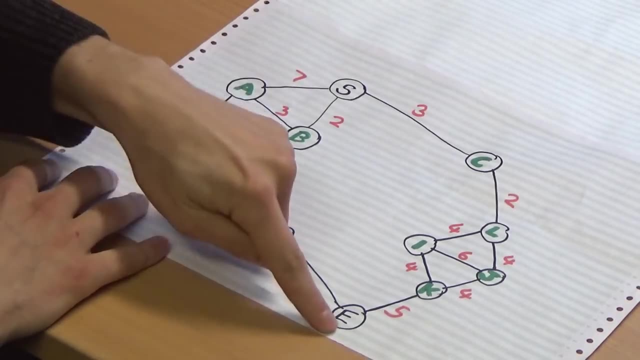 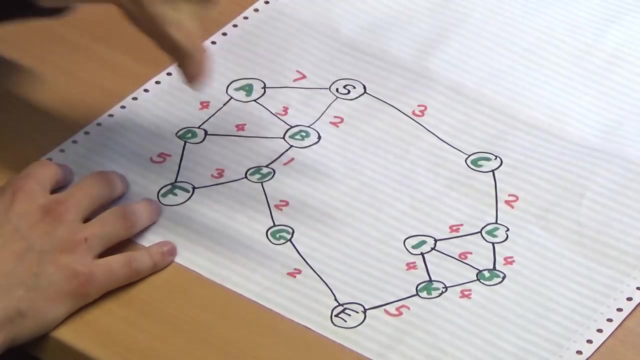 So in the Dijkstra implementation that I am familiar with, and most Dijkstra implementations, the smaller is better. So, broadly speaking, this route here is kind of like our motorway Twos ones. that's good. This one is a bit of a faff, you know. fours, maybe middly A roads. 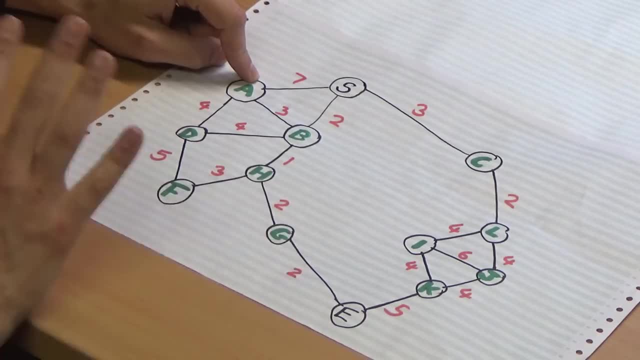 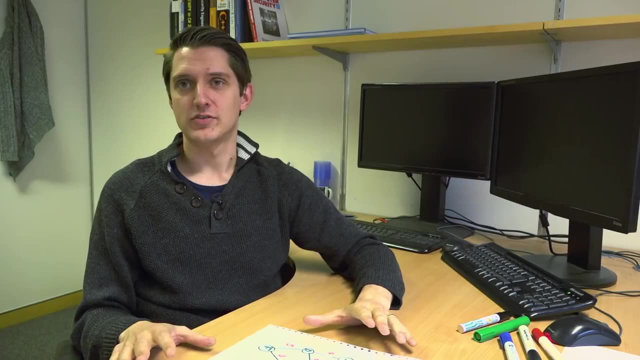 And this seven here. that's you falling in a ford and you've got water in the engine and it's bad. The question is: how do we find a route from here to here? Now, of course, this is a small graph. 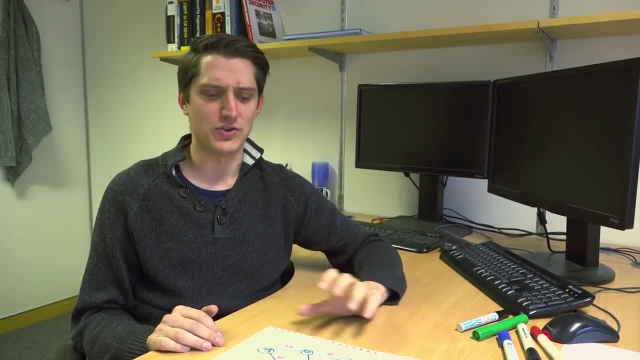 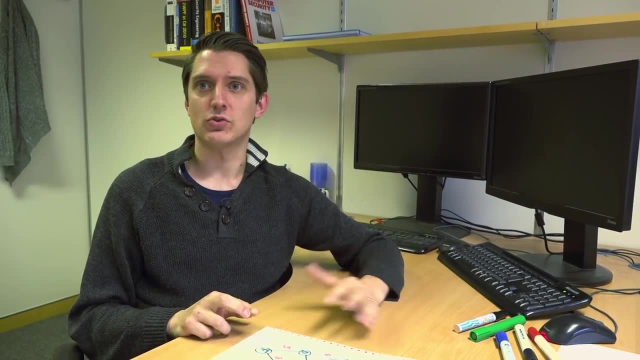 So actually what we could just do is just search all the way through it by hand or using a very simple sort of brute force search approach And kind of get the best go right. But if you think of the UK or the US or some other country's massive road network, 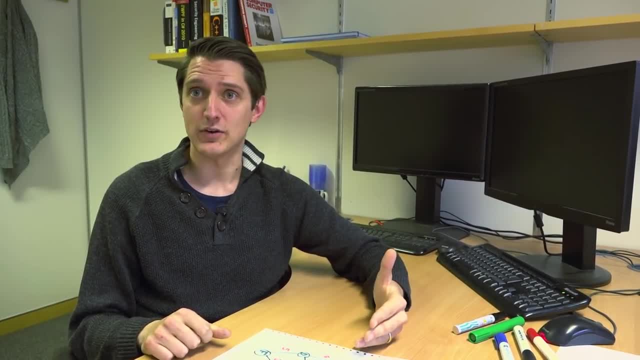 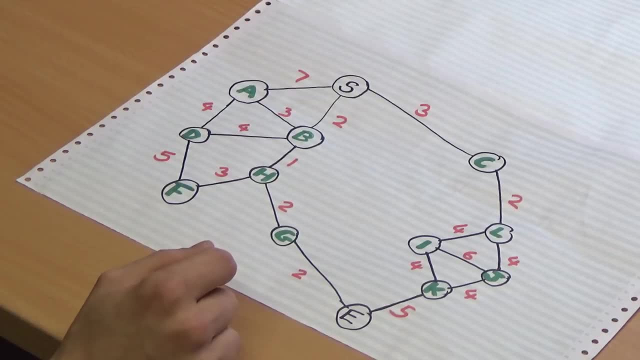 we can't afford to do that right. We have to be a bit smarter about how we look through, And we also want to know absolutely that once we found a route, it is in fact the shortest route and we didn't just miss one. 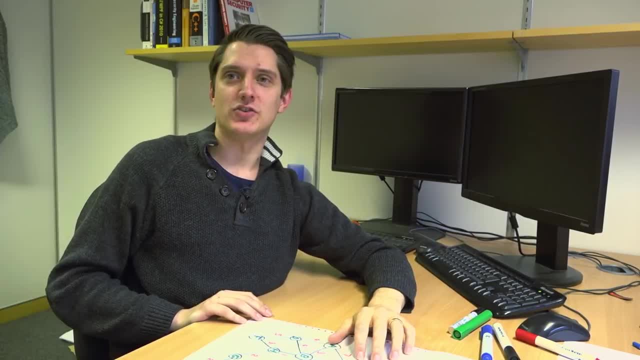 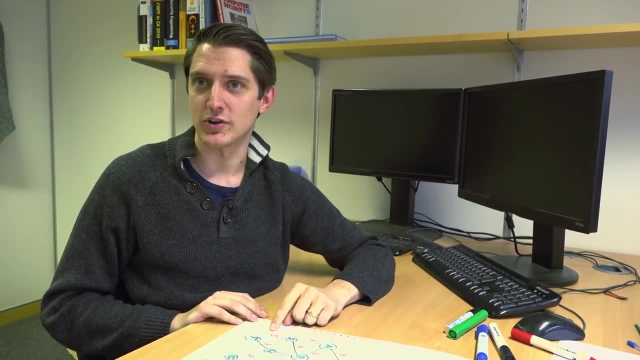 What Dijkstra does is basically similar to a sort of brute force flood fill search through this space, but does it in a kind of in the order that makes most sense, based on how fast these roads are. So we'll check the quickest roads first. 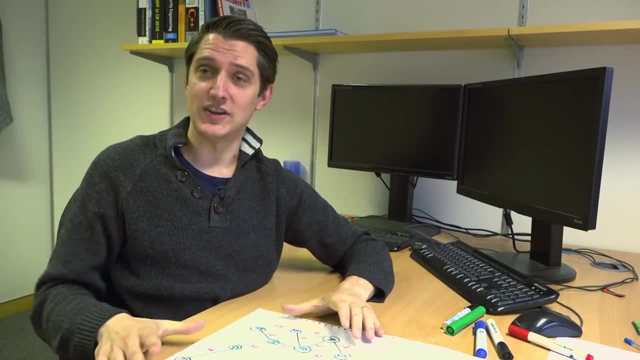 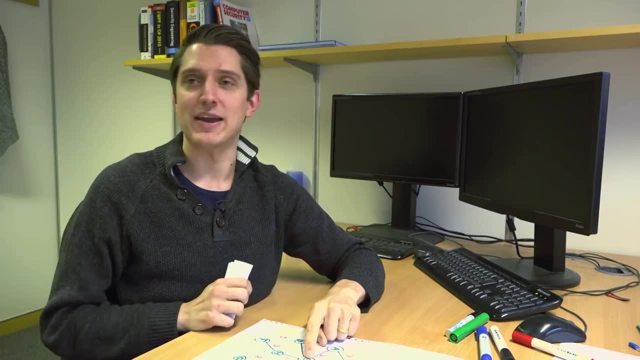 So to do Dijkstra, we need a few things. First of all, we obviously need our graph right And when. we need some idea of how long the path is to, let's say, B once we've calculated it, or something like that. 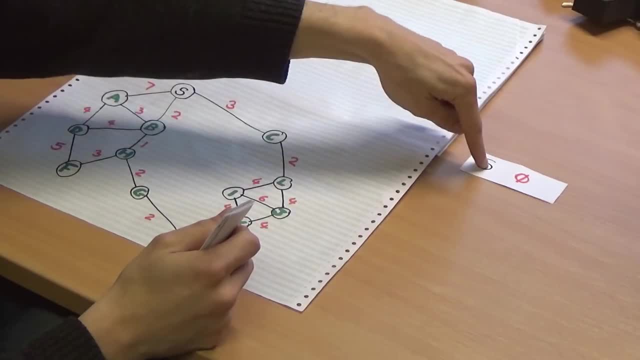 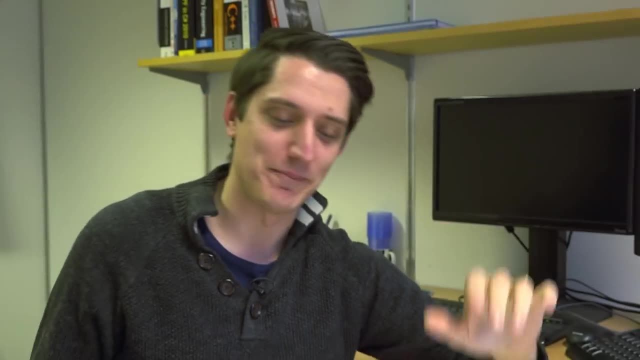 So at the very beginning of our search we have S. We are at S, S for start right, S for start, yes, Which confused me because some of the other letters are just in order and then these two aren't. But anyway, S has a distance of zero right. 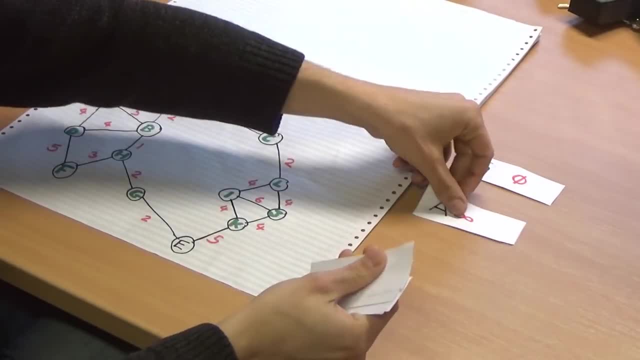 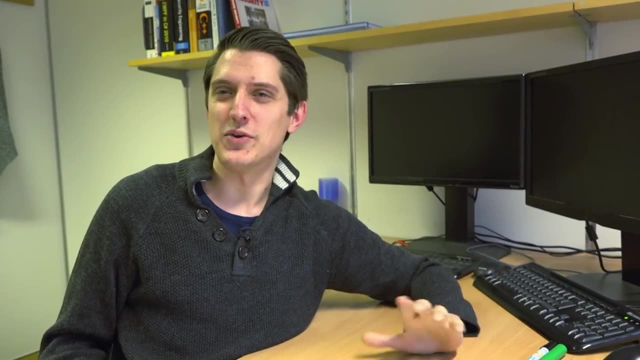 It costs me nothing to get to S because I'm already there. The first thing else I'll just put a couple out just to show you. A, B and K have a distance of infinity, because that basically says we haven't looked yet. 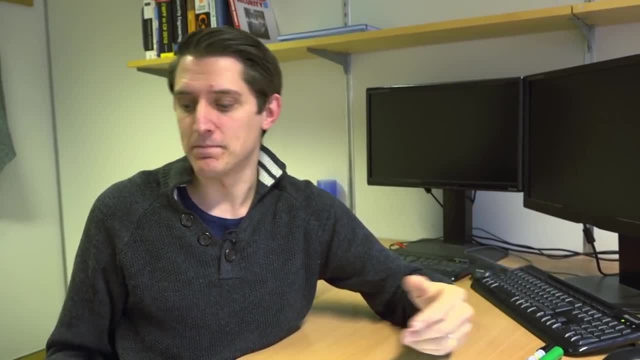 We don't know how far, So, for all we know, it might not be possible to get there right. And finally, E is just the same distance of infinity, but with a smiley face to say that we've made it right. 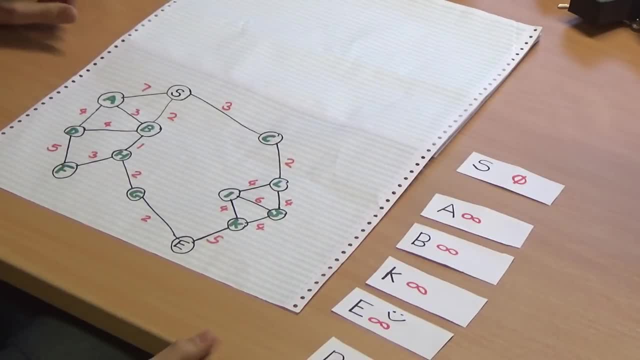 Now, this structure here that I'm going to create is called a priority queue. Each of these will have a distance, but they're ordered also by that distance, So the shortest ones at the top. that's important, And we'll do it as we go through. 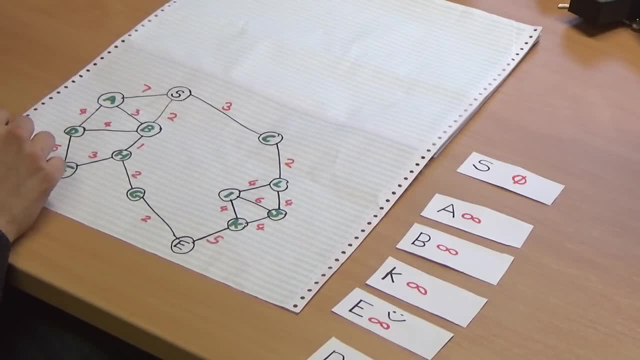 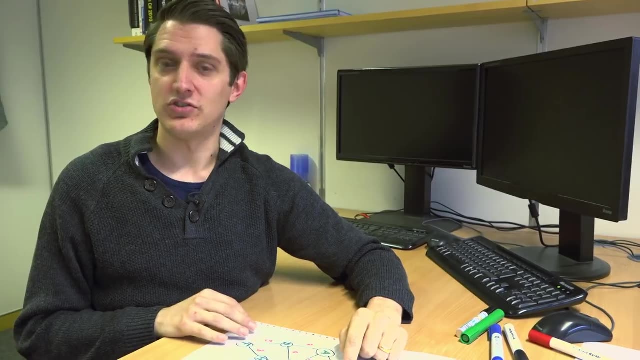 So let's start our search. We start at S and we look through the neighbors of S And we say, right, well, A, it cost me seven to get to A right. It's a bit of a pain. So we were at zero distance cost of seven. so now we're at seven, right? 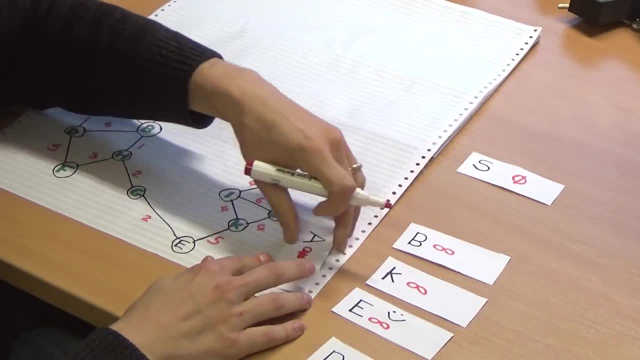 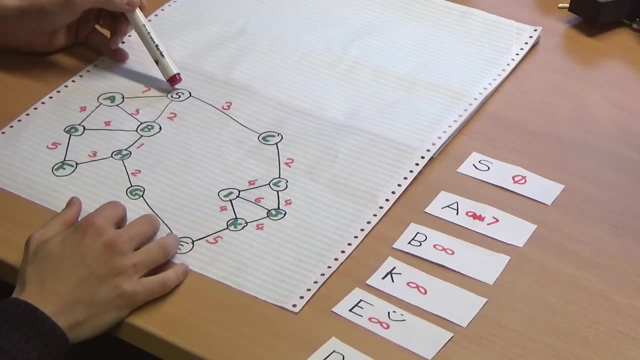 So A, I scrap my infinity and I write seven, right, So A is seven. okay, A is still the second shortest path currently, because all the others are infinity. yeah, B is zero plus two, so that's two. So let's just put a two in there. 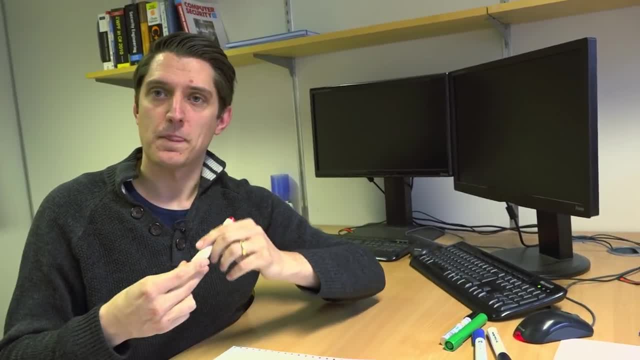 This is all, even though we haven't actually got to the end yet. You're just looking at the numbers. We can't get to E without having a look through all of these junctions. So this is what we're doing, and we're working our way in a smart way. 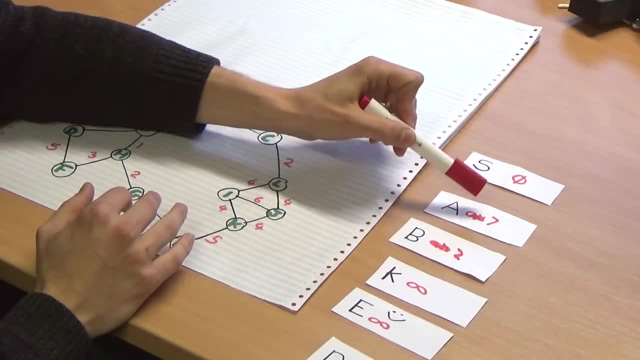 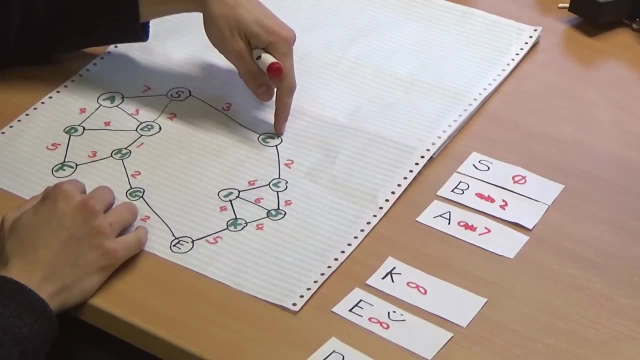 Now, B is in this priority queue, but it has a lower number than A, So it takes its place at the top of the line. okay, So that's good so far. Finally, the only other thing connected to S is C, which has got a weighting of three. 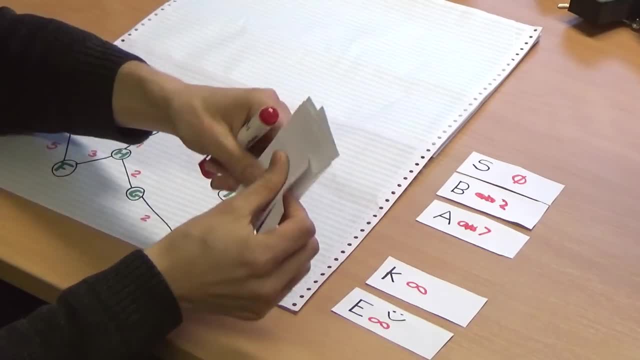 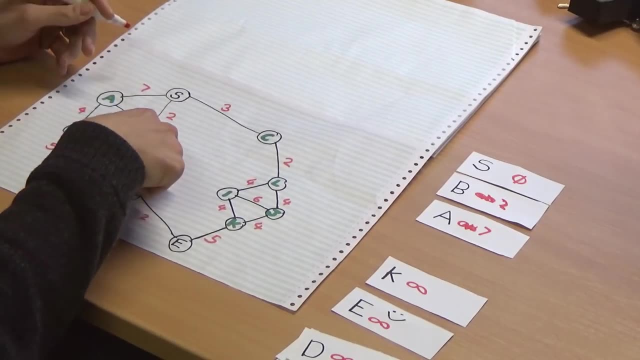 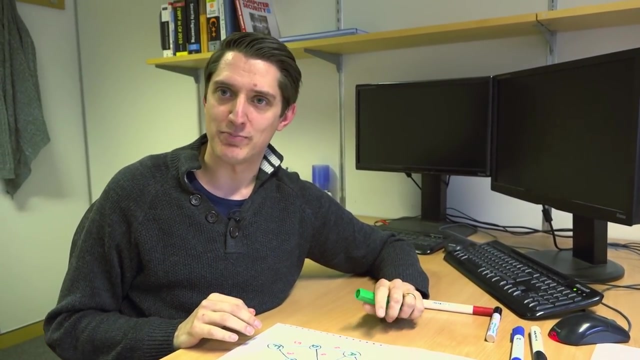 So let's just find C in my list of, of course, shuffled thingies. There we go, And hopefully how dikes will work will start to become clear once you see what I do next. So C is three. The only other thing that, of course, I forgot is, while we're doing our search, we have to keep a track of where we've been. 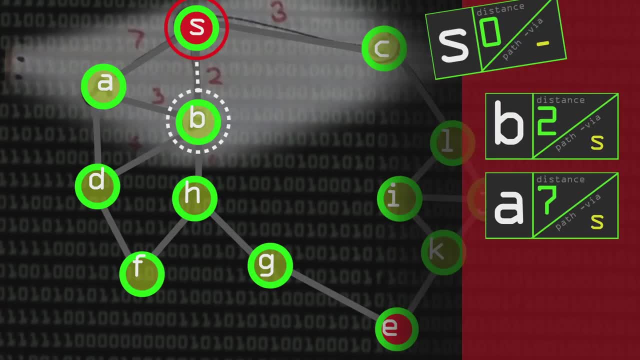 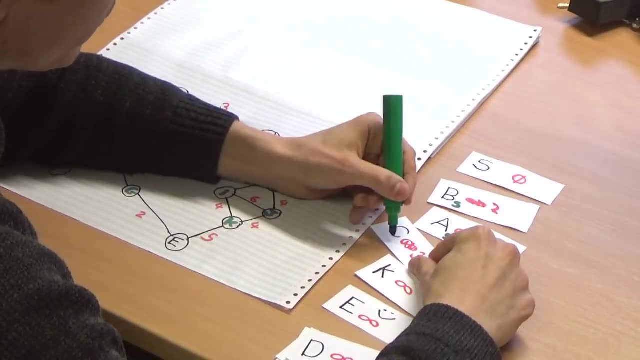 So B, for example, we know has a distance of two through the path S. okay, So S was the previous version, right? That's also true of A and also true of C. Now we swapped C and A, so now we have them in order. 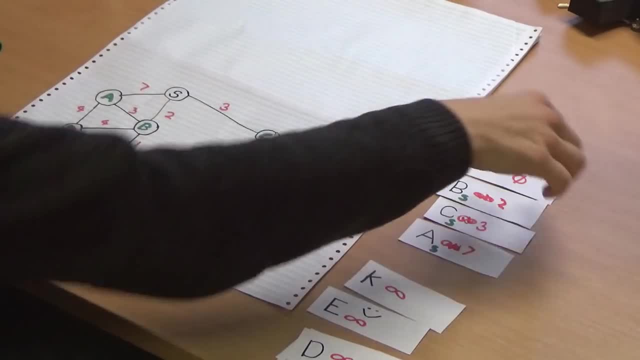 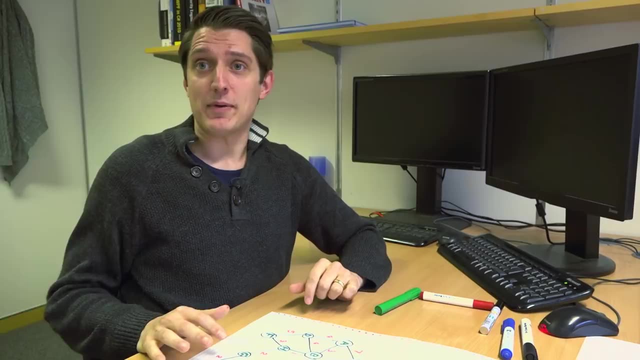 All the others are still infinity. Now S is done right, So we can take that. We can take S away and put it in our finished pile over here, right S we don't need to worry about anymore. The next step is to see where is the current shortest path. 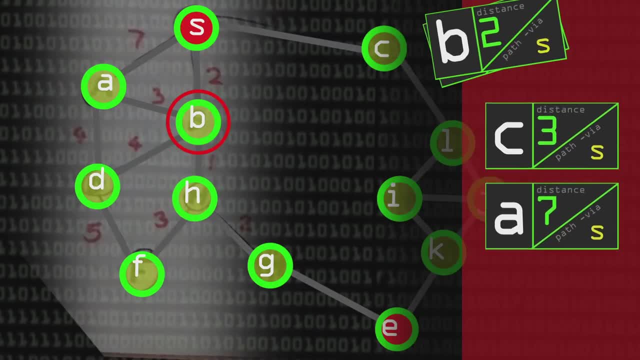 Well, it's B, right? B's got the lowest number, so let's start looking at B. So if we look at B, we've already been to S, so we ignore it. We can go to D, so let's put in a D. 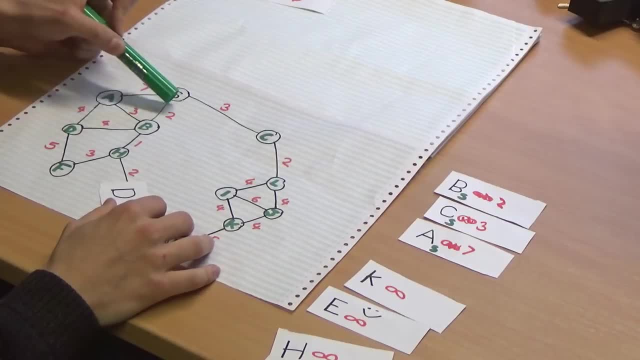 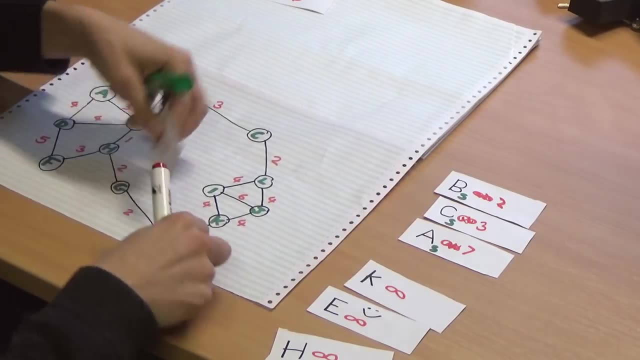 And D is the distance to B plus whatever this road is, which is six. Two plus four is six, And the route through D, which is shortest, is currently going through B, And we'll put that in Now. six goes in just above A. 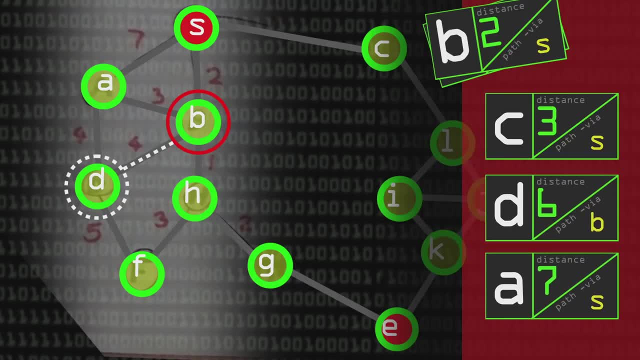 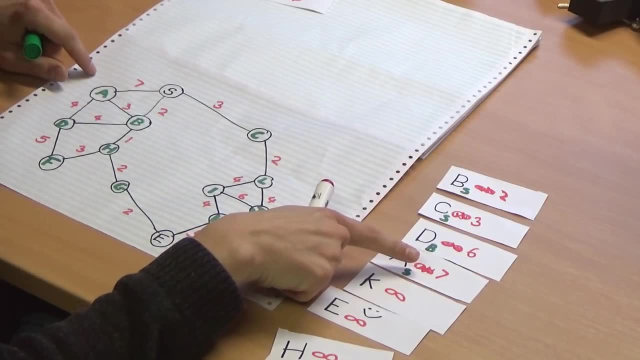 Okay, there we go. Now we can also go to B from A. We haven't finished with A yet. It's just sitting in this queue And currently the distance to A is seven. right, But actually the distance to B was two and the distance to A from B is three, which is five. 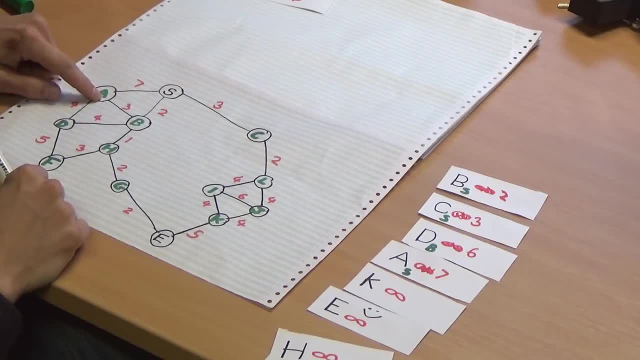 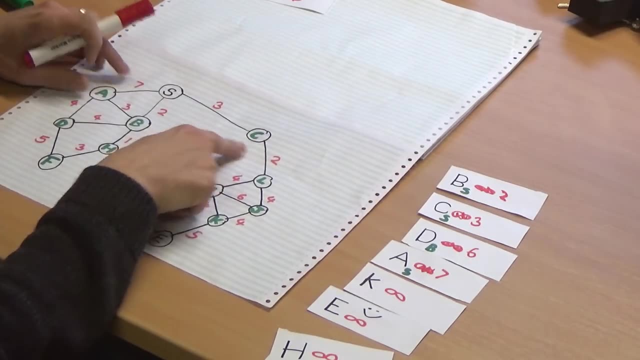 So actually taking this detour here, which looks longer, is actually shorter because of this tree on the line or something like that, right? So remember, you know this isn't representative of the actual physical distance from S to C, So we've updated D. 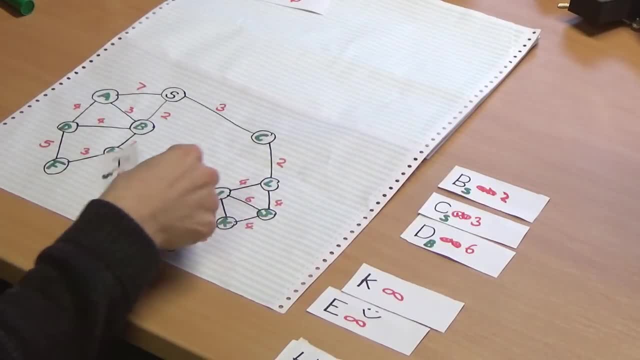 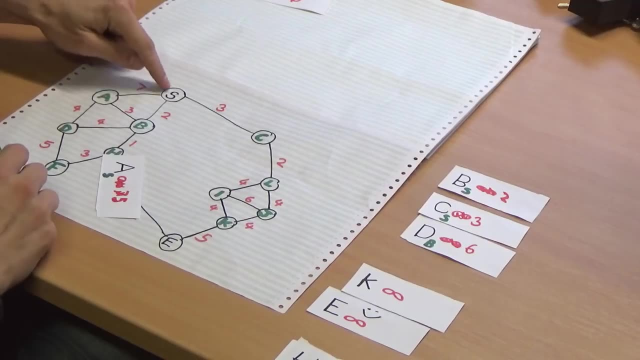 And A is now shorter, right. So we take our A and we say, well, now the route is five, not seven, It's decreased And it's no longer the shortest path from S to A, It's from B. 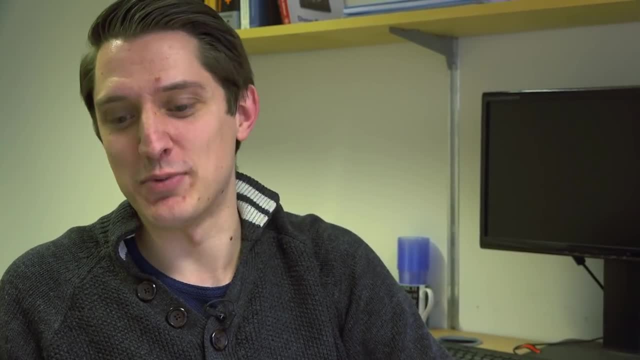 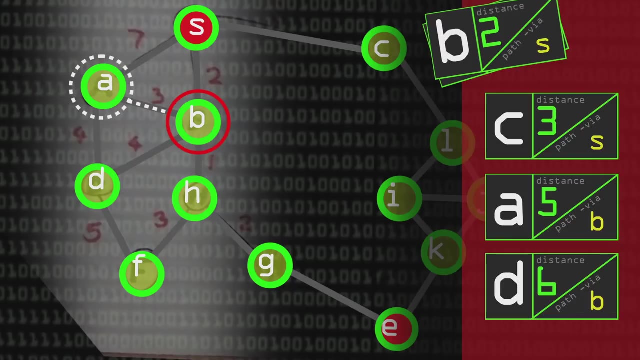 So we can scribble out S right? I'm getting too much text on these, but we won't worry about it. So A now overtakes D in our priority queue, right? So that's looking good, Okay. H B had a length of two. 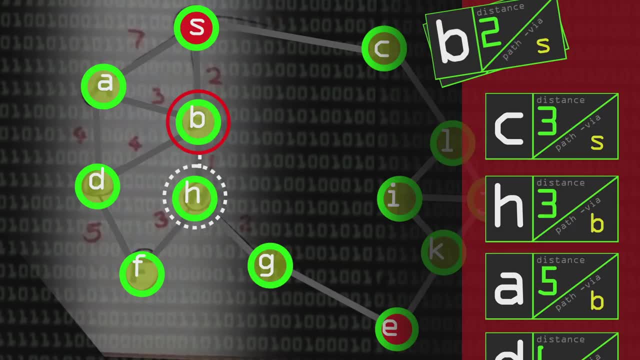 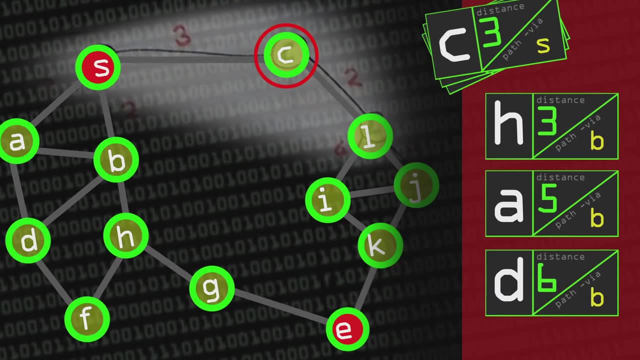 H has a length of one, So H has a distance of three. B is done. right, We've done B, We can count that as done. So C next right. So we're here. We can't go to S. 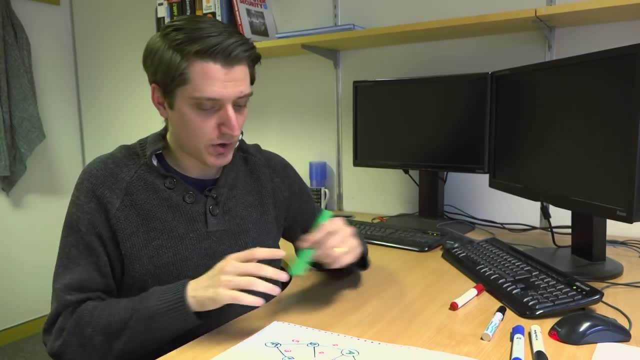 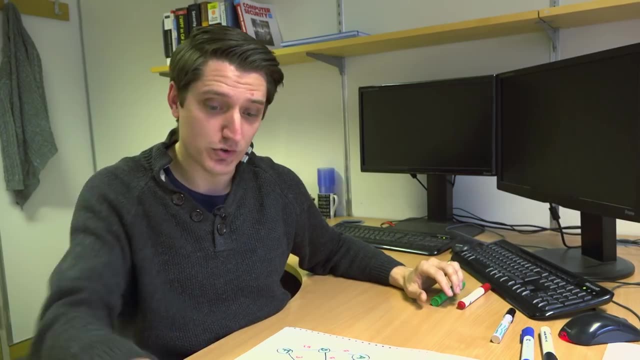 We can only go to L. That's a nice easy one. So I need to find L. So L goes to C And it's three plus two is five, So L comes in just underneath A like this. So C is done. 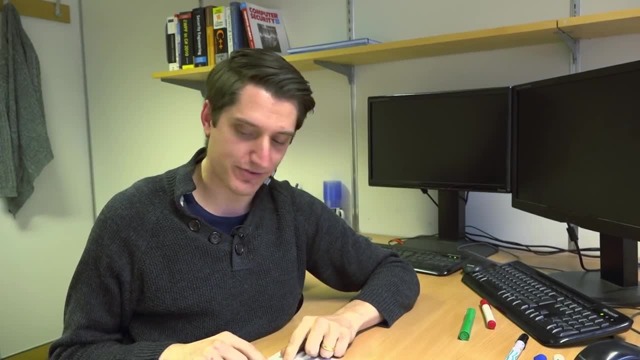 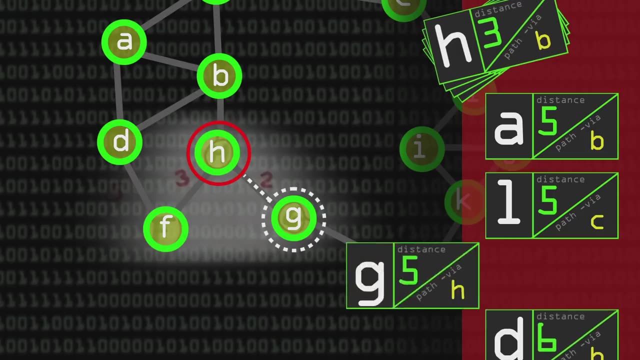 So we look at H and we say: what's next from H? We can look at F, So F will get three plus another three, So that's six via H. And then G is H, which is three plus two, So that's five. 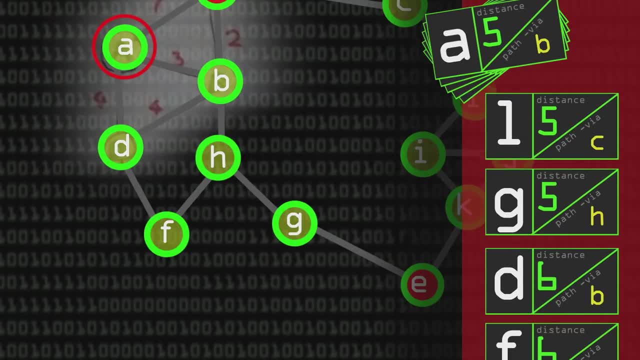 A. next, We've already been to S, We've already been to B, So we can start to get a little bit faster now. We've seen some stuff already. What we're basically saying is: we know what the shortest path to B is, because we've already seen it. 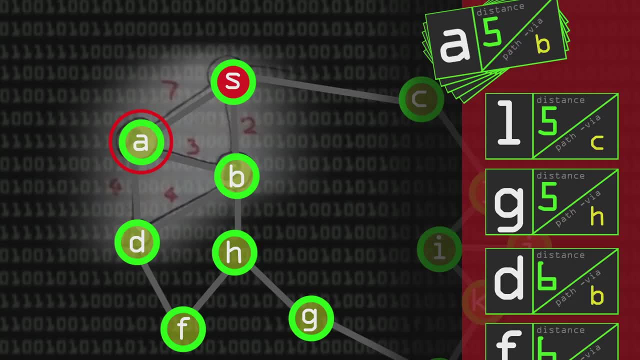 So we can only look at new things. So we look at D. D is currently six via B, A is currently five. Five plus four is nine, which is bigger than D already is. So we make no change. The shortest path to D does not go through A. 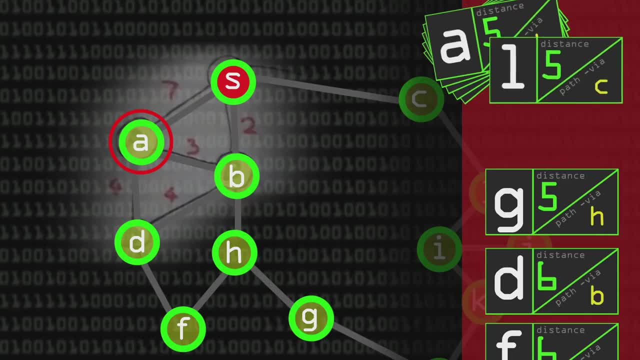 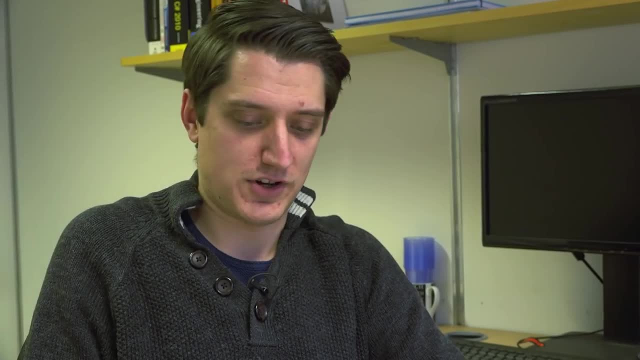 So we don't worry about that. Okay, A is done. L- L can't go to C. We've already been there. I and J both have a length of four, So let's just find those. I and J Nearly done all of them. 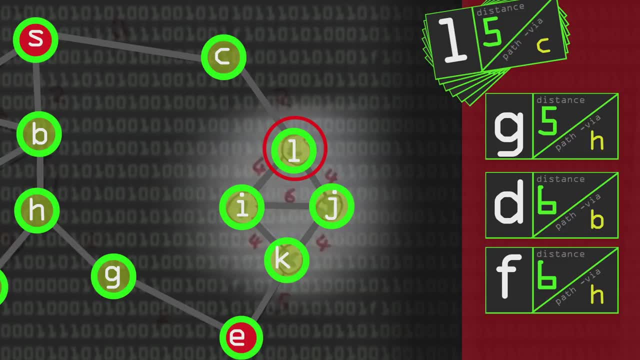 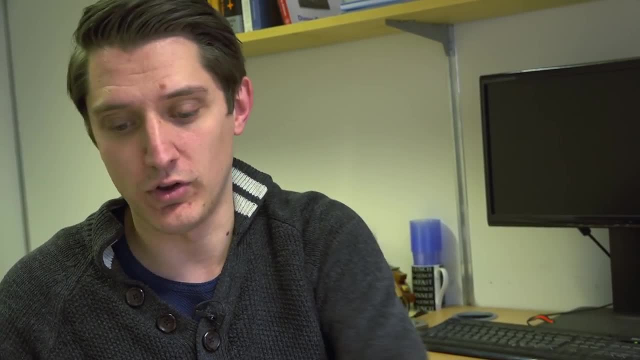 Right, So these both go through L and they both have a path length of nine. Nine. Okay, So these go, and they're both long, but they go in front of all the infinity ones, but down at the bottom here. 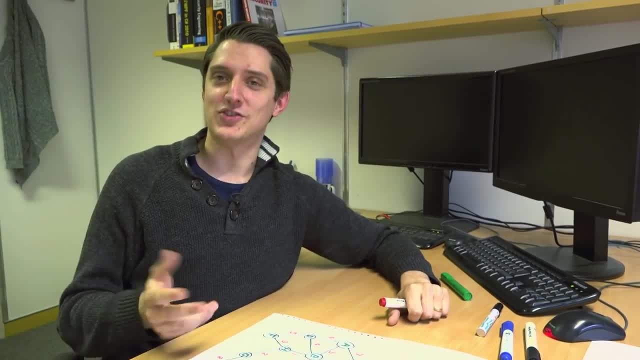 All right, The order isn't important. So how are we doing? L is done, So then you can see what's about to happen. Right, G's got a distance of five. We've already been to H, Let's go to E. 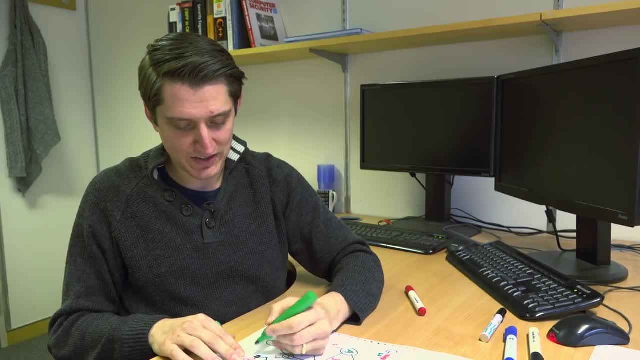 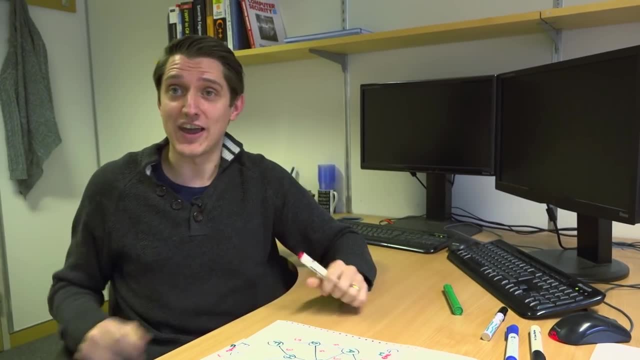 And so we say E goes back to G and has a length of five, six, seven, And we're there, Right, And then the final step is just to backtrack our route based on where we've been. So E goes to G. 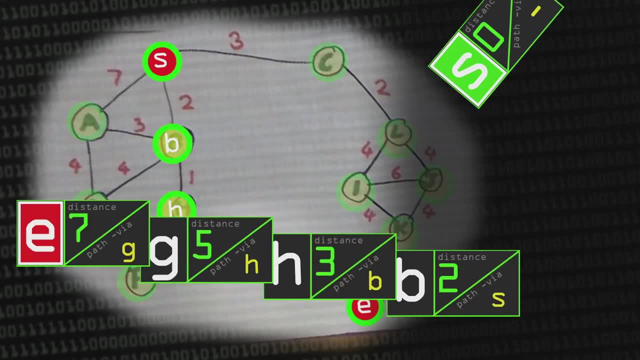 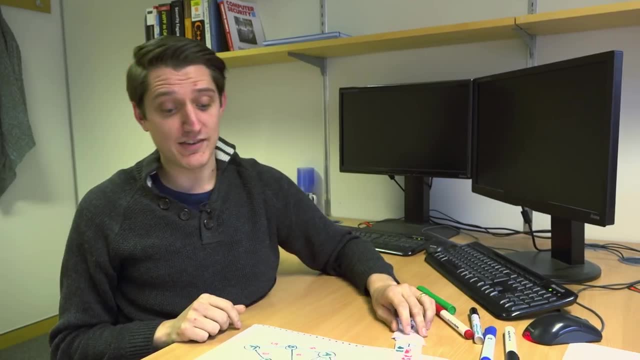 We can skip these that aren't used. G goes to H, H goes to B And B goes straight to S, And that is our shortest route. through this graph as found by Dijkstra, The idea is that if this graph were much, much bigger, 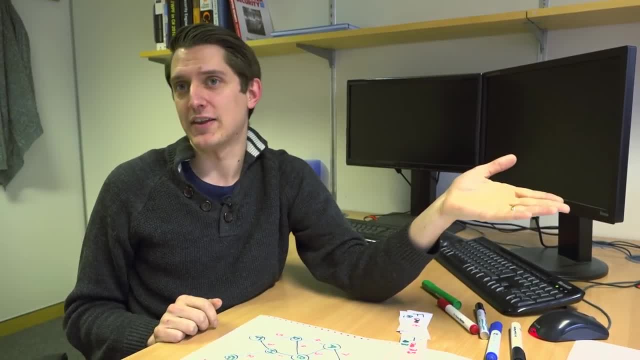 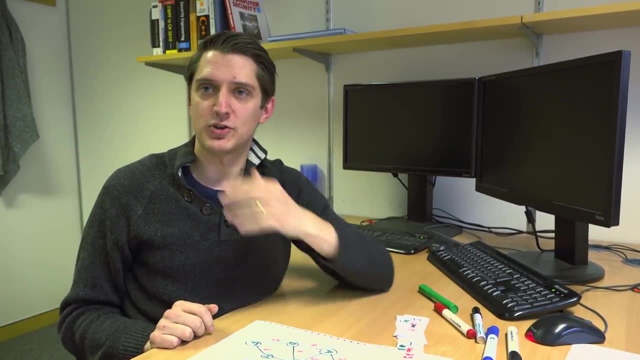 you would prioritize looking down motorways first because they have less weight, and you would prioritize physically short distances, anything that you can to try and make your search a bit quicker When you're searching to, let's say, travel from Nottingham to London. 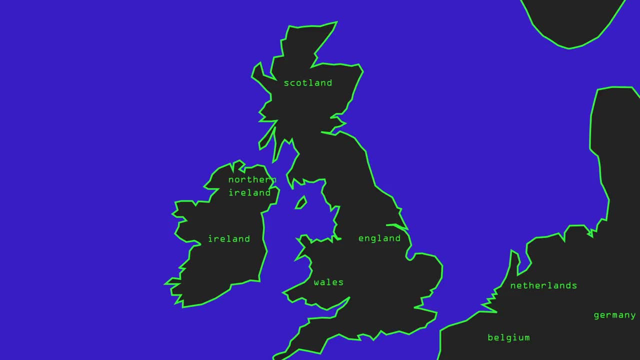 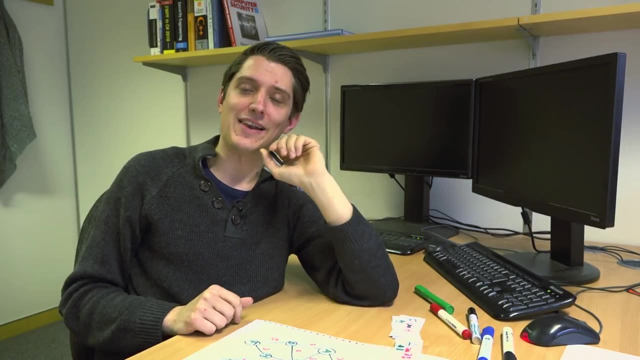 you don't look at the roads- in Scotland, at least not first, because it's unlikely they're going to be the shortest ones- What you do is you get yourself to the M1 and start traveling down towards London as quickly as possible. That leaves us with one last problem with Dijkstra, which is perhaps for another video. 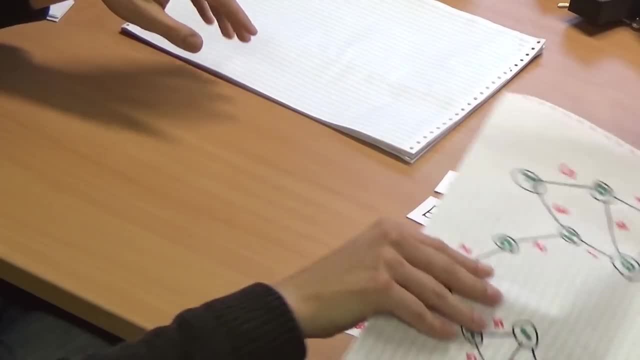 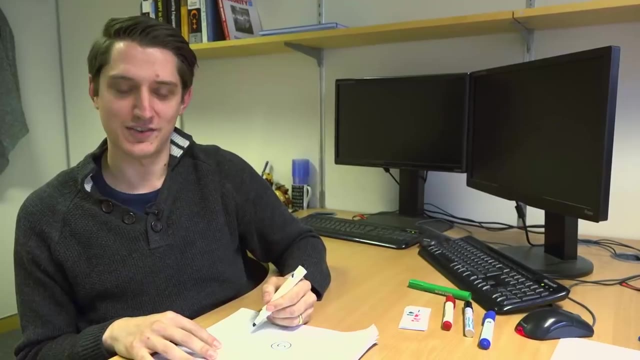 but I'll just introduce it. If you imagine a situation where I'm at my house and, let's say, my house is here at an S and this is sort of M1 junction right, which happens to be about junction 26,, but we'll call this A right. 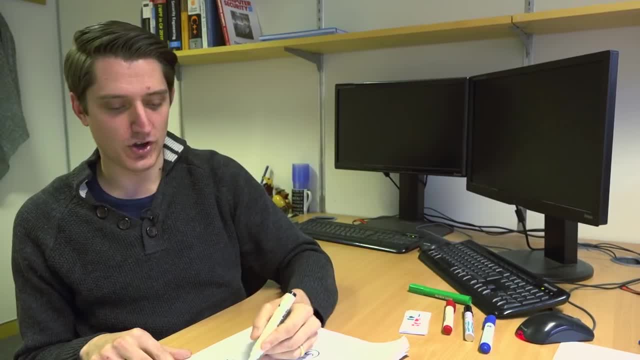 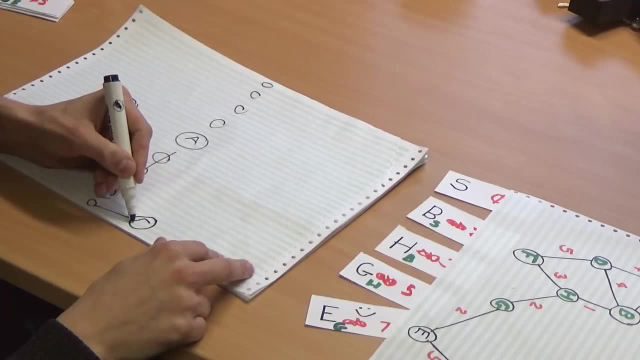 And then this is where I'm going in this direction. so lots of nodes along here and there's lots of nodes along here And this is my destination, down here, on the end of this motorway, Because of a slight traffic jam. these all have slightly higher weights than these. 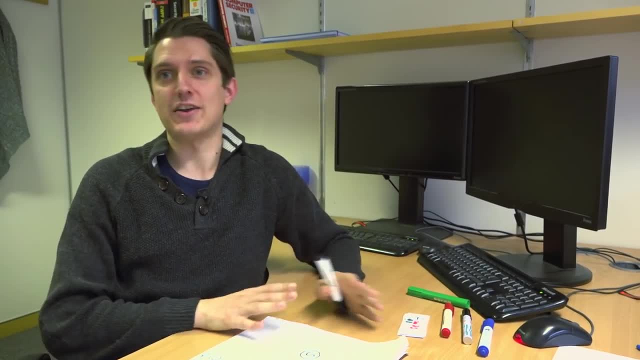 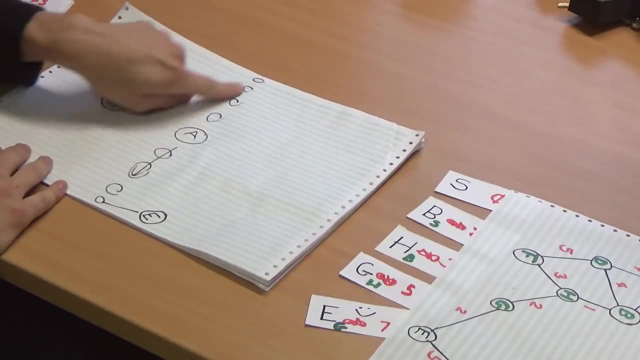 Because Dijkstra doesn't build any idea of the direction you're traveling, any kind of heuristic about what you're doing in a sort of smarter way. it's going to look up here first. It's going to travel all the way up this motorway as far as it can. 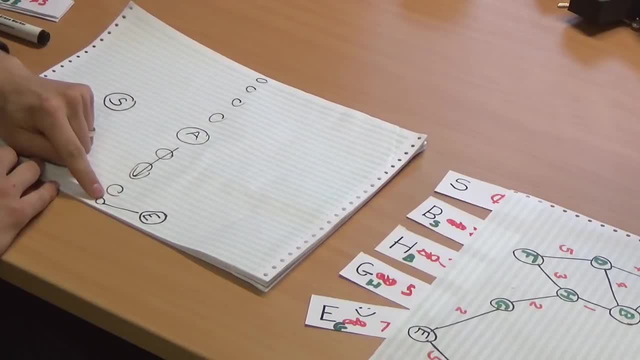 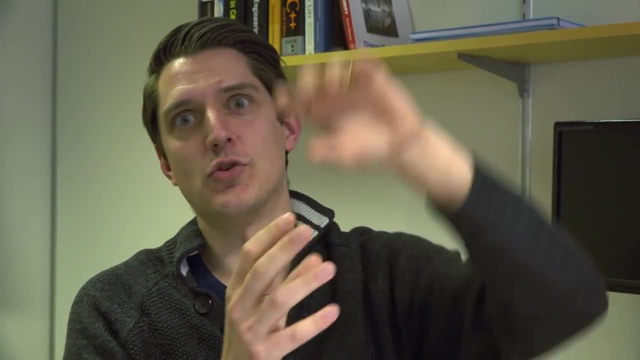 and only change direction when it becomes the shortest path to do so. So what you need to do if you're going to actually implement a sat-nav is be a little bit smarter. Don't start sort of looking to all the fast roads. Look at the fast roads that are going roughly in the right direction. 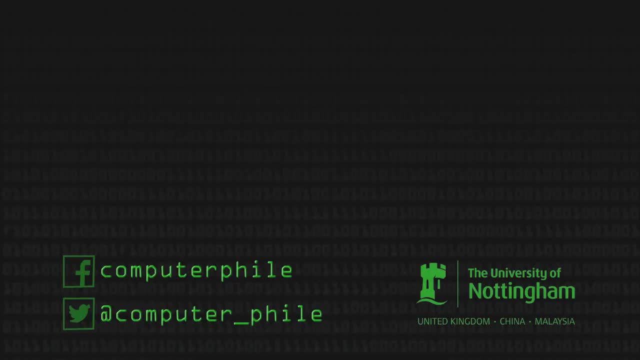 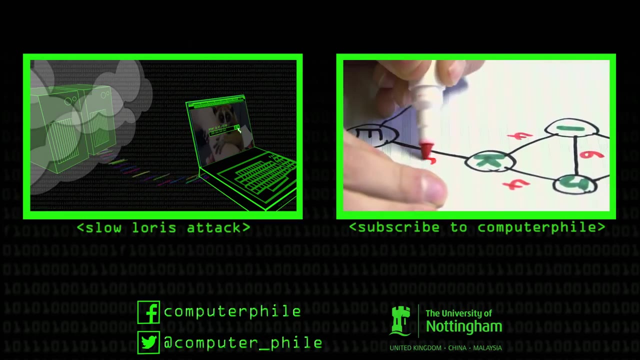 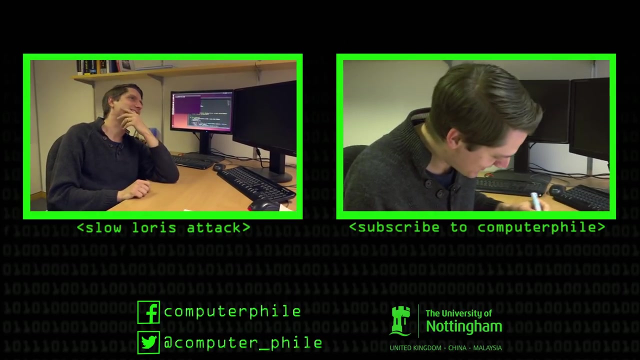 because otherwise you might be wasting a lot of time. And then red, Why not red? Right, I think I've got them all, E I think E's got to have a little checkered flag on it, doesn't it? Well, E Yeah, well, how do I draw a checkered flag? 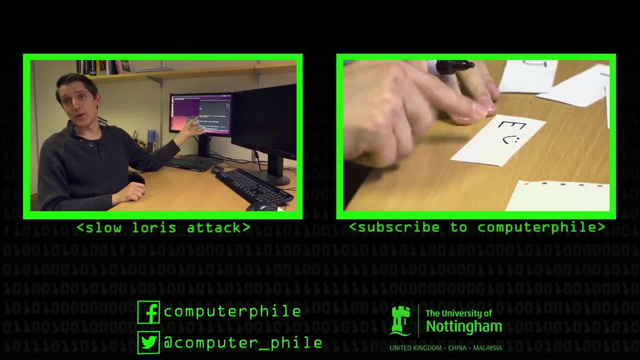 Smiley face: All right, That means we're done, Right, okay?